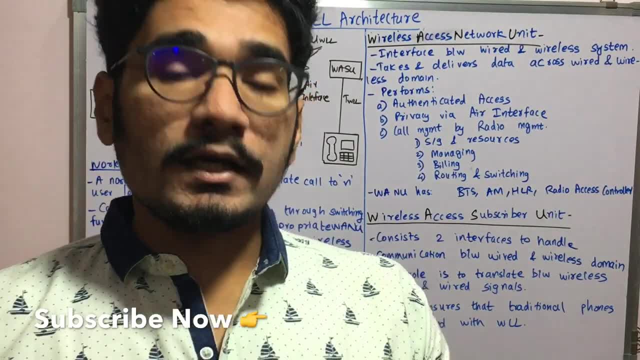 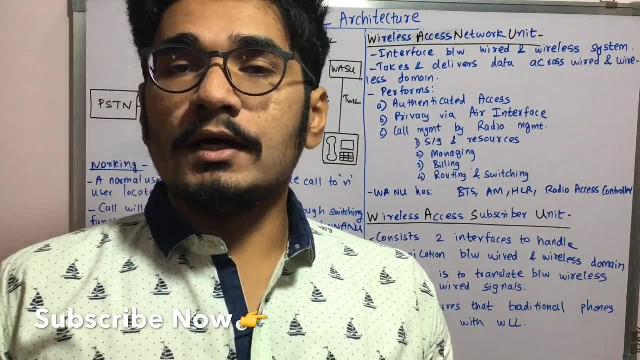 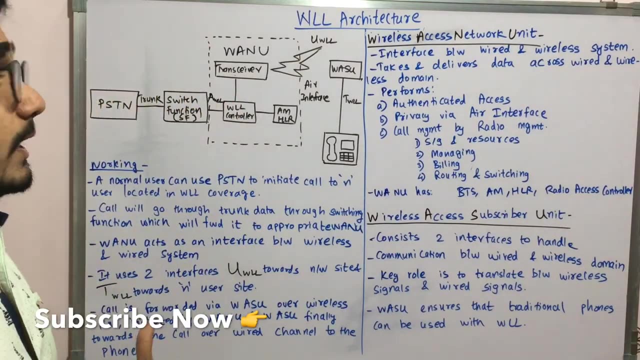 Hi guys, welcome back to my channel. So today in this video we will see the architecture of wireless in local loop, that is, WLL. So in our previous video we saw why WLL came into existence in the wireless technology and how its significance is there. So in today's video let's see how the architecture of WLL looks like, or what architecture does it possesses. So to begin with we basically start with the diagram. So this is a diagram of how the WLL looks like. 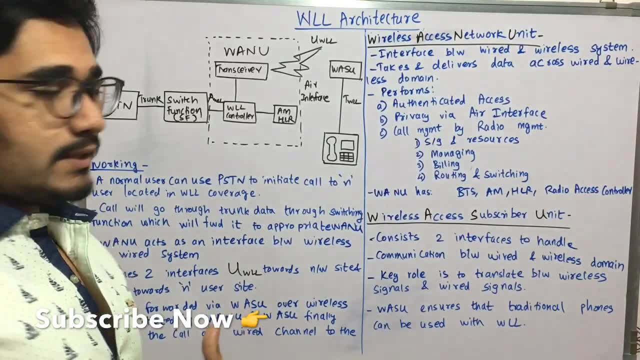 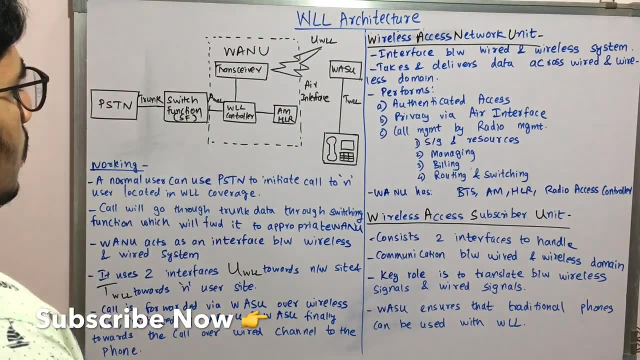 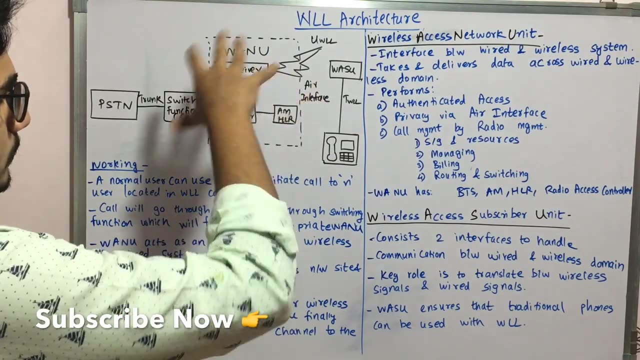 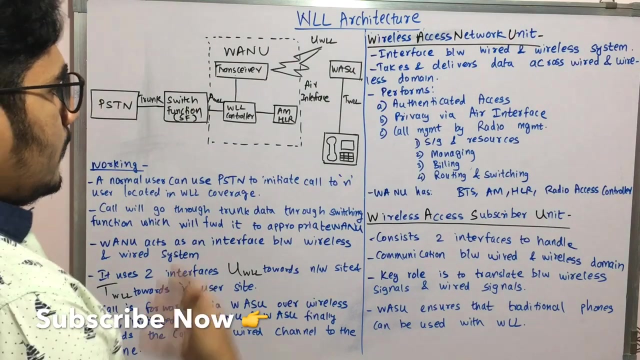 So it has got few components. So it has got the public switch telephone network PSTN and it is connected to the switch function SF via a trunk. Then we have a unit called as the wireless access network unit, VANU, and it has got few components. It has got trans receiver, it has got WLL controller, it has got an access manager AM, it has got the home location register and which are all wired connected. 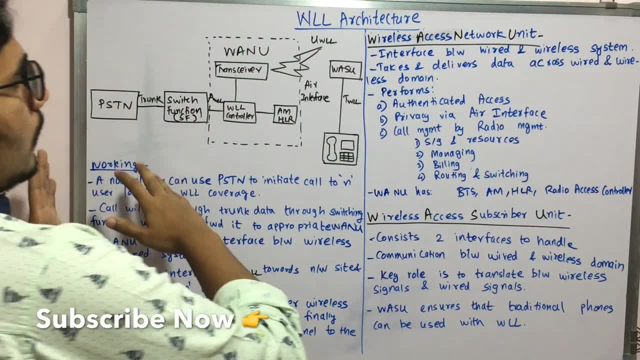 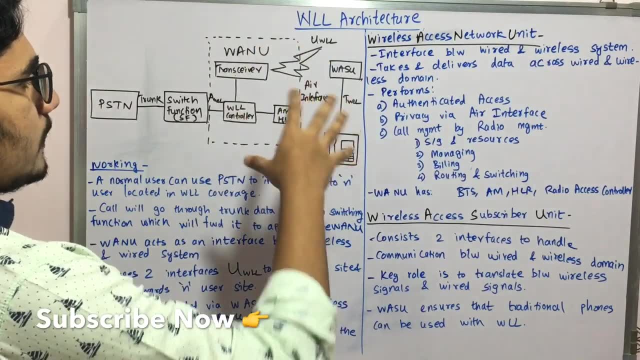 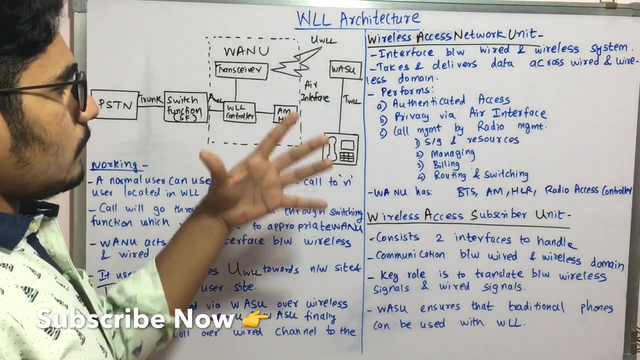 in this architecture are all wiredly connected. now, when you come to this side, that is, towards the right, you have everything wireless. so everything here is connected by means of an air interface. it's called as UWLL, and so you have a unit there also. it's called as the. 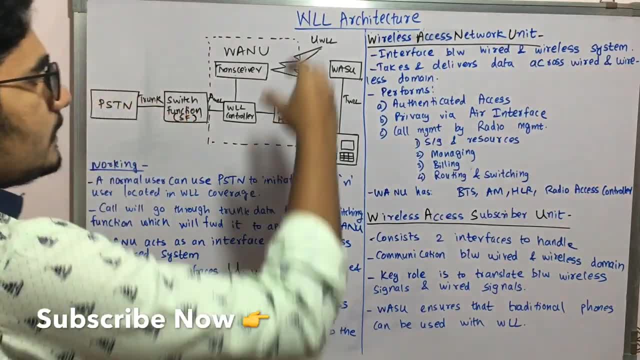 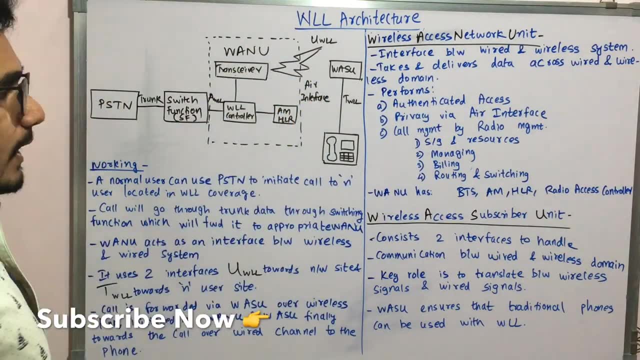 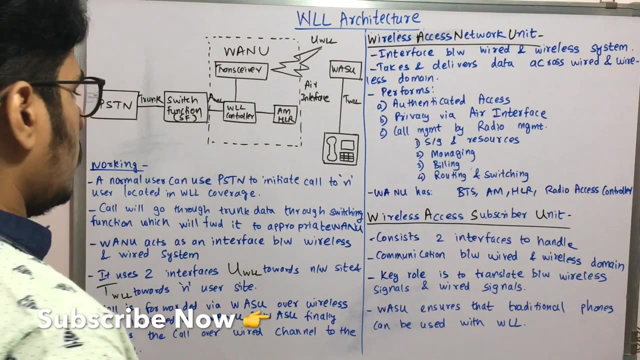 wireless access subscriber unit, VASU, and then it is connected to the telephony systems or to the end user via TWLL. so that's another wire which is connected. so let's see the working or how the call routing takes place in WLL. so basically normal user can use the PSTN. 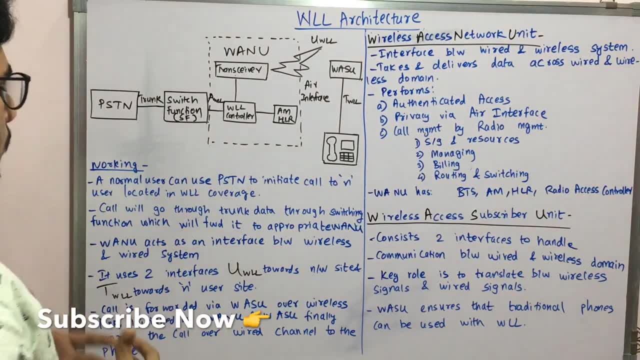 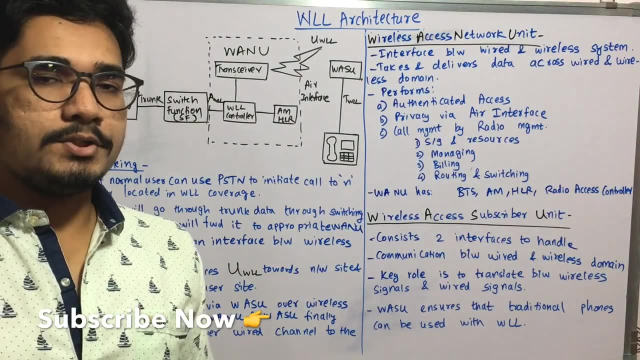 that is, public switch telephone network in order to initiate call to end users which is located in that particular wireless coverage area. so it's like in your locality or in your region you may be connecting to different people with different networks. so in this case, you may be connecting to different people with different numbers. so that's what PSTN. 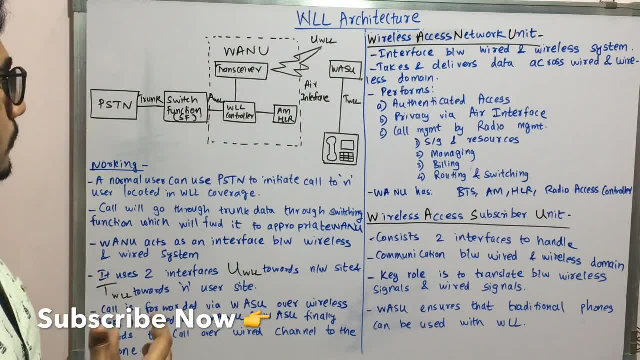 is so in WLL, in order to initiate or in order to originate a call, you can use the PSTN. next call will go through this trunk data. so call will be routed through this and through switching function, that is SF, it will forward to appropriate VANU. so basically, this VANU changes as in. 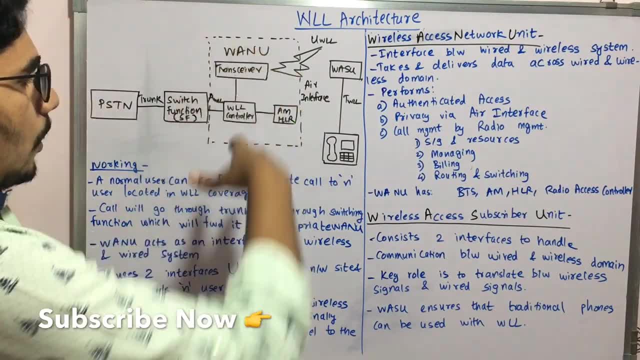 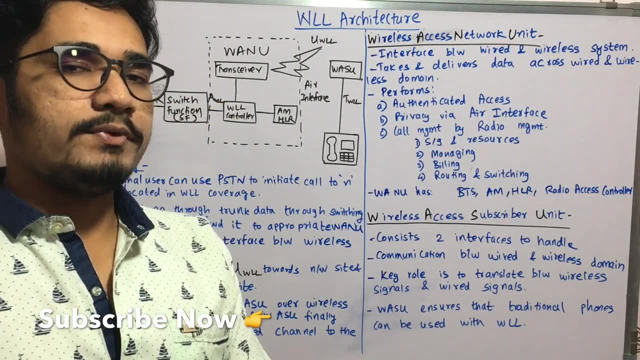 when the requirement changes for the end user. so here the components which you see that is in this. So the components which you see that is in this, So the components which you see that is in this selects. So basically, if user requirement changes or the head office demands that you need to. 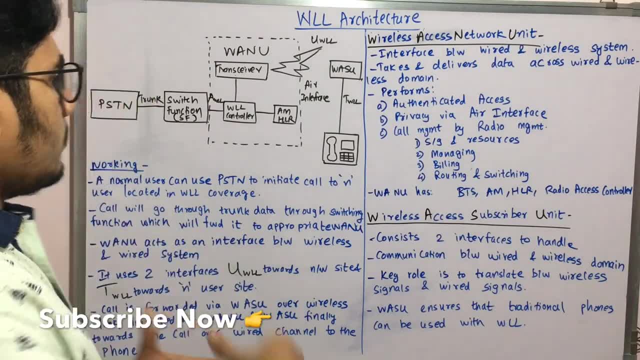 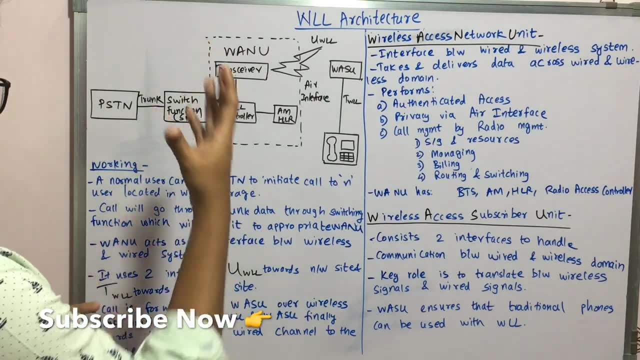 install these many components inside the VANU, then there will be some additions or deletions inside the setup. so I know here access and interface between the wireless and the wired system. so whatever you see on this left side is the wire towards your right. you will have. 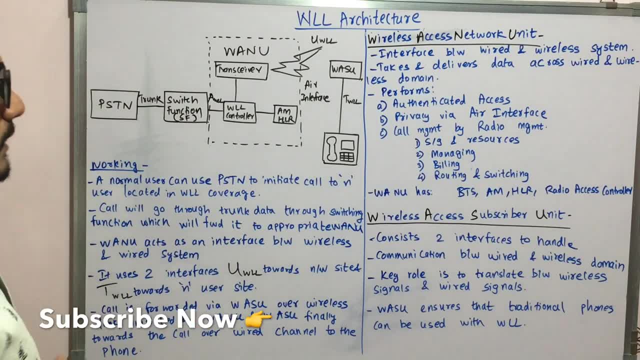 a wireless system, so it uses two types of interfaces, as you can see: UWLL, which is connected, connected towards the network side, that is, which are accessed wirelessly, and you have TWL, which acts towards or which connects towards the end user side. Next call is forwarded here via VASU and over the wireless link and it's initiated by VANU. 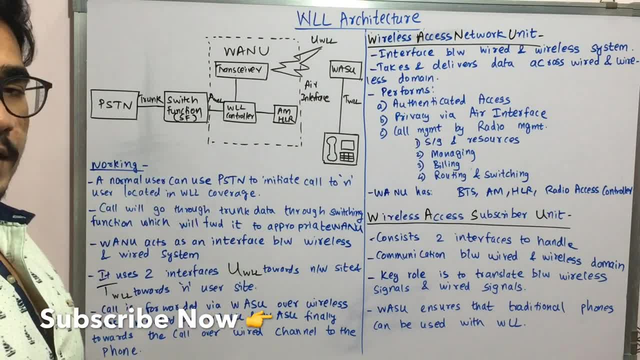 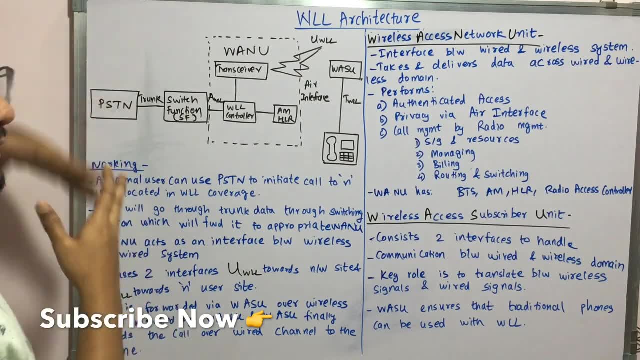 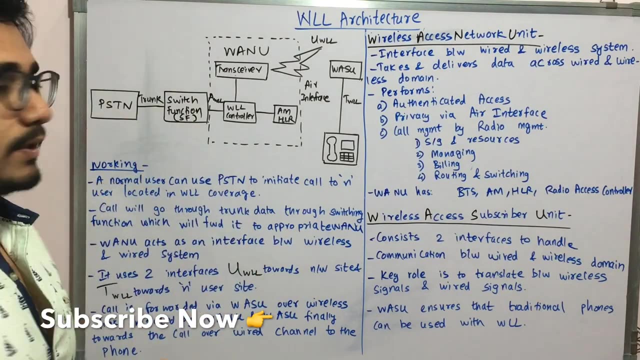 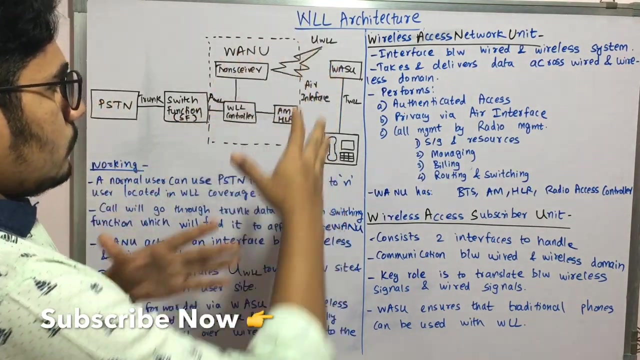 and VASU and finally towards the call is transferred over the wired channel phone. So whenever call just is initiated it passes through the trunk and then switch function has an algorithm or it's intelligent function just decides how the call has to be routed and which all components has VANU got and then accordingly it will just route through. 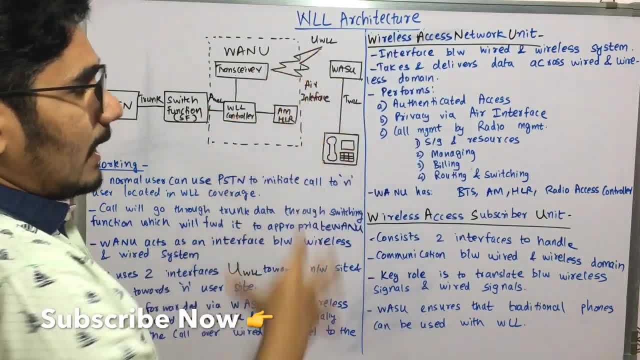 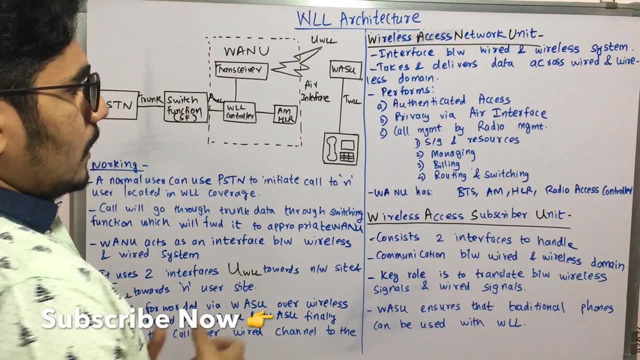 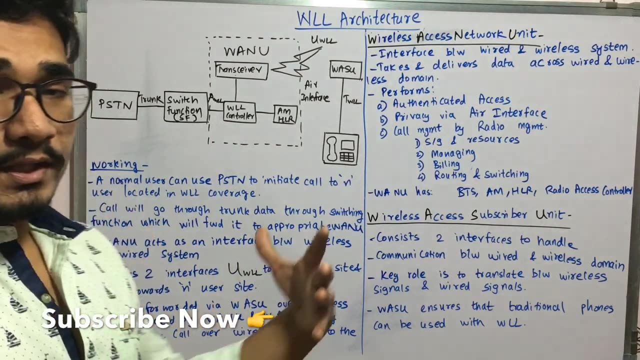 the air interface and then at the end system you have the wireless access subscriber unit and through that medium of wire at home you may be having that wire. Thank you, With RJ45.. So with that user would be getting a call. So now this is how the architecture or the working basically of WLL is. 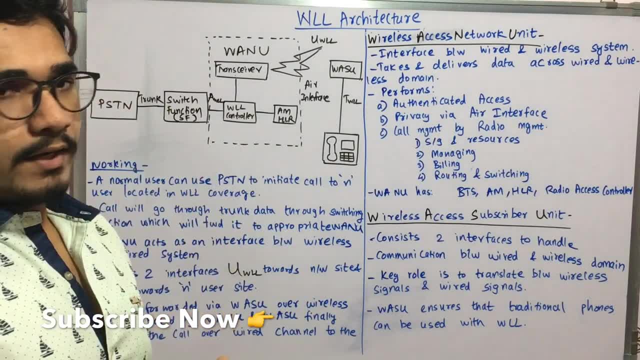 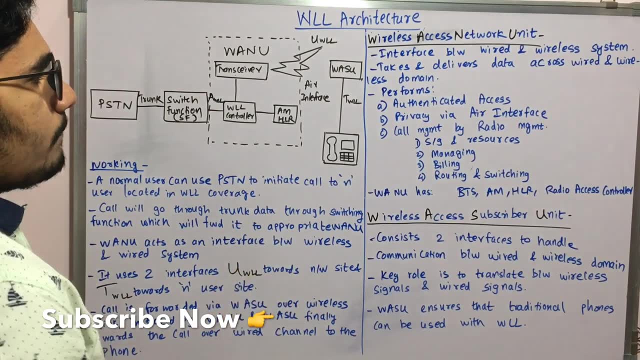 Now let's move on to the two prime components in this, that is, we have the VANU, that is, wireless access network unit. So it basically acts as an interface between the wired and the wireless system, like we saw, and it basically takes and delivers the data across the wireless domain. 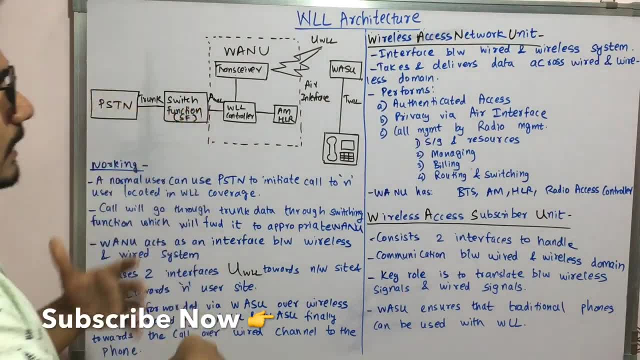 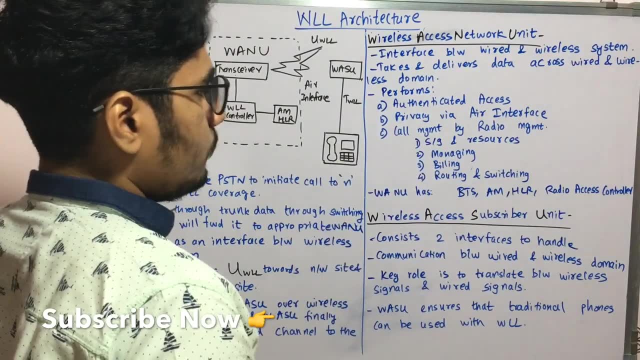 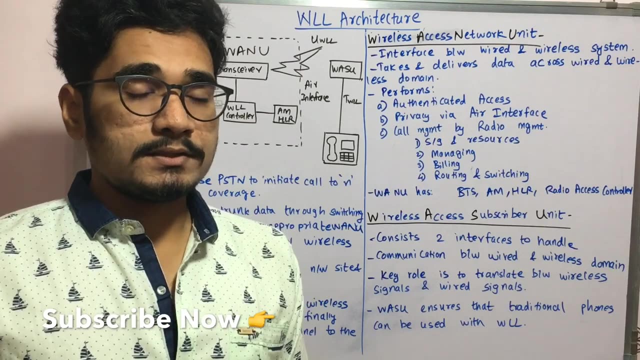 So from here it takes the data. whenever user makes a call, it takes the data And then it is distributed over the wired and the wireless system So it performs you a couple of activities. So those are authenticated access: So whenever user is dialing a number, so it checks whether that particular number is complied. 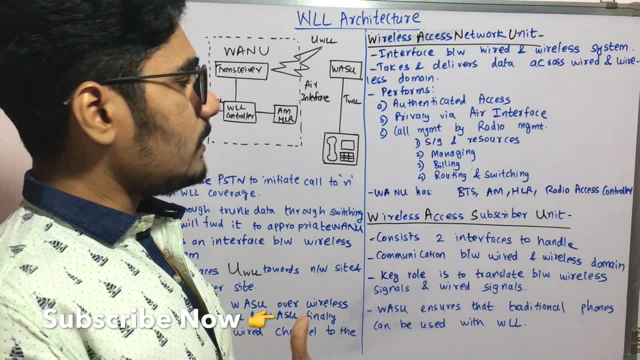 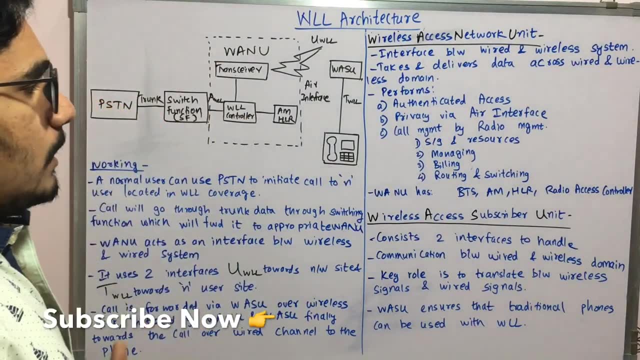 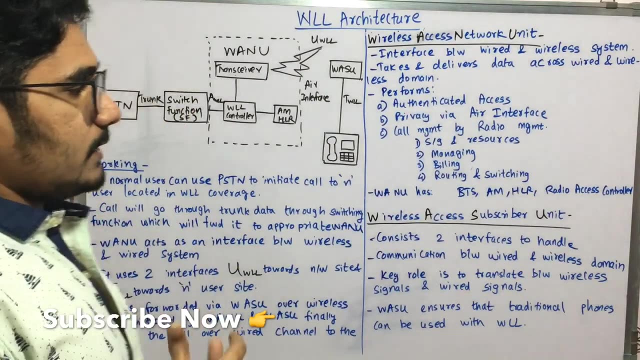 to their standards. Then the privacy or the call security is maintained over the air interface. That's very much important and call management is done by the radio management. So this setup has got a few of this. It has four different parts, that is, it basically deals with the signaling and the resources. 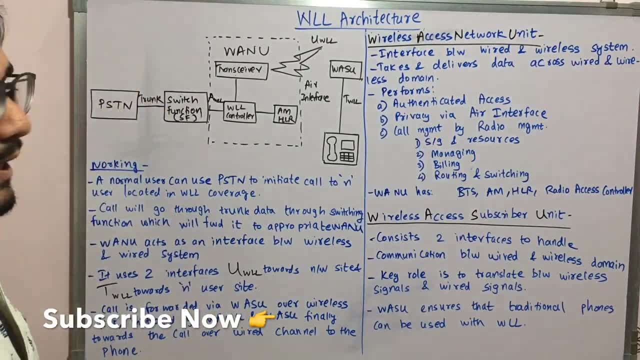 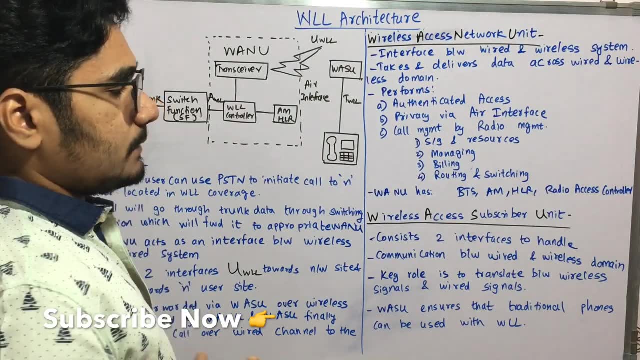 Then all the managing and billing, routing and switching- everything is managed by the VANU And VANU has few of the components like. this trans receiver is basically your BTS from the GSM system. that is base trans receiver station, And then you have the AM. 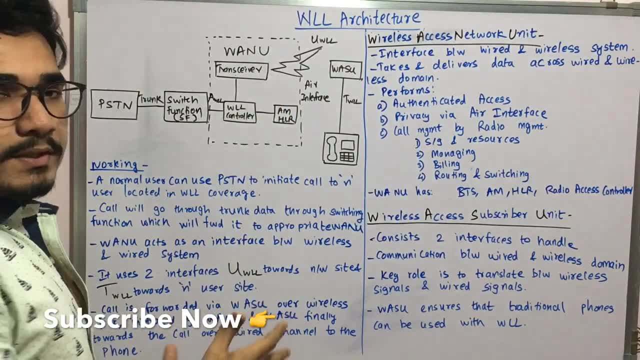 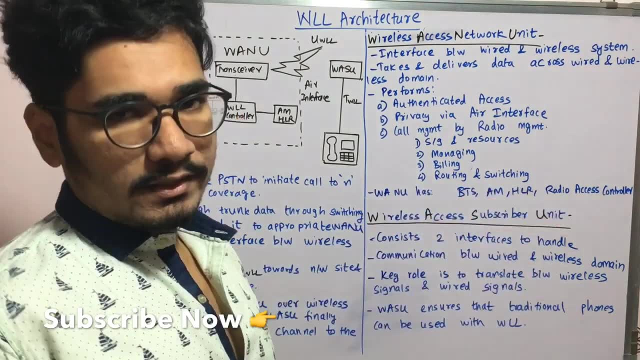 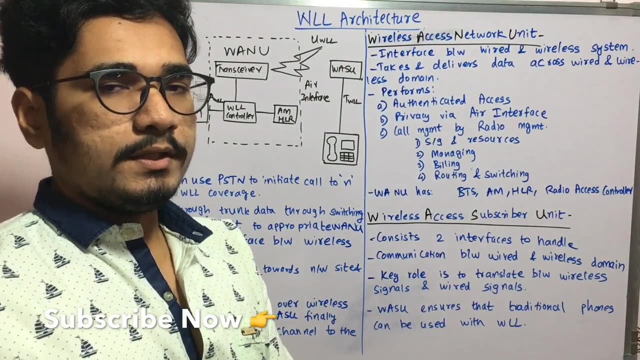 So AM you can find here, that is AM, HLR- AM is access manager, which is used for security purpose. Then you have HLR, that is home location registration. Then you have a radio access controller. that is an optional component which is there, So that controller basically just controls all the functions or the calls which is coming. 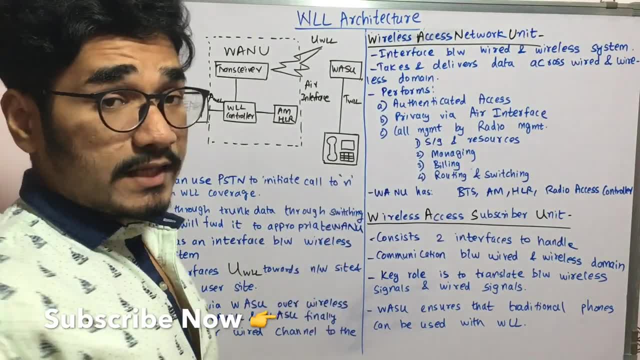 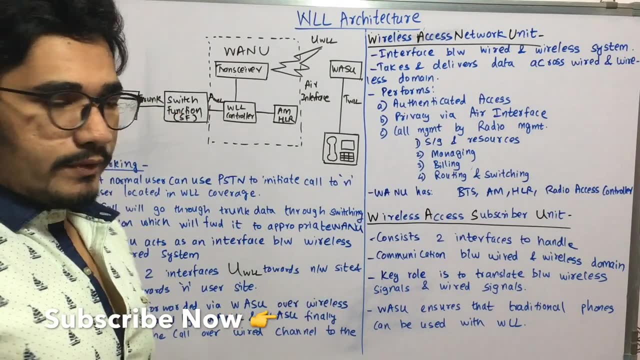 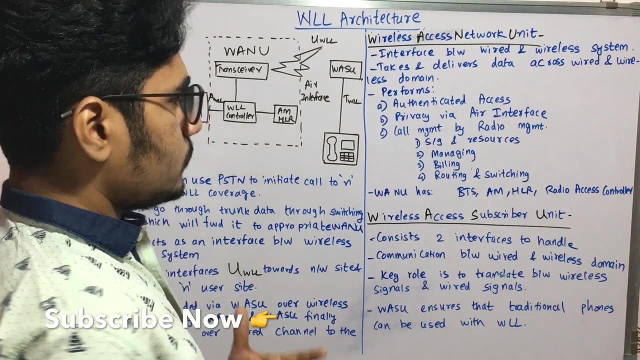 through this. Next you have the wireless access subscriber unit, that is, this part which is in the wireless domain. So it consists of two interfaces basically to handle. So the communication is made between the wireless and the wireless wired domain. So those things are handled by the VANU. 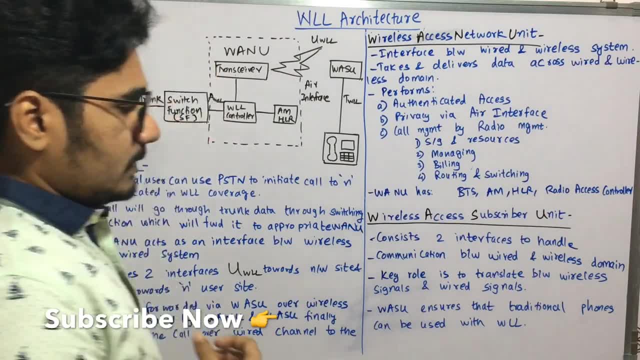 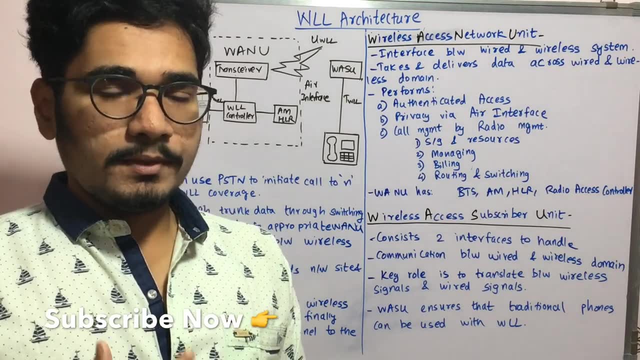 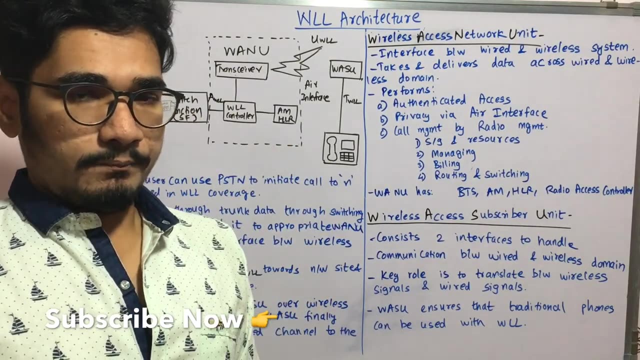 And the key role of VANU is to translate between the wireless signals and the wired signals. So whenever the data is coming, so it will find the appropriate encoding mechanism and then it will translate into the wired system so that it can, or the end user can, understand. 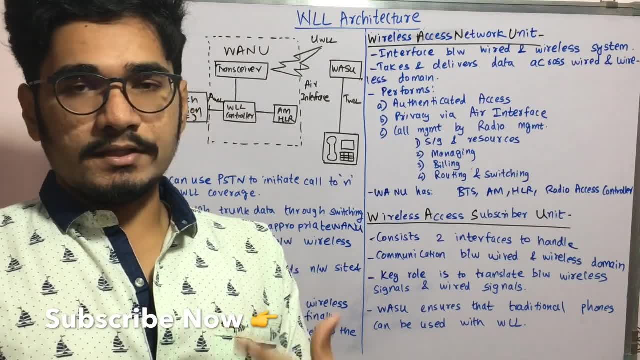 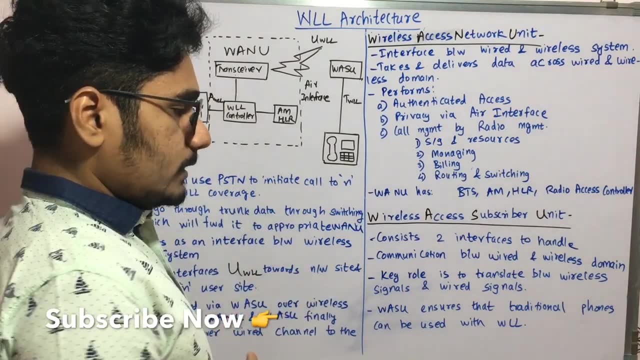 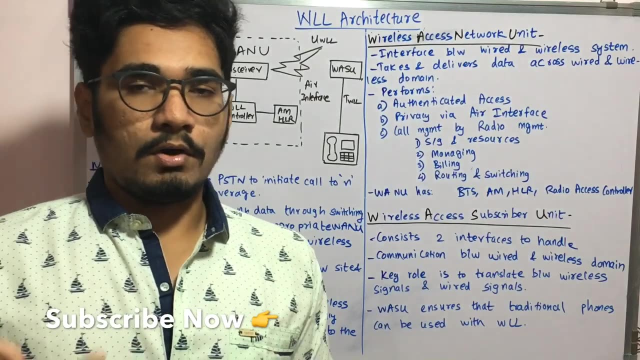 what's being spoken, whether it's a text message or whether it's a voice message. So basically it translates those signals into appropriate forms. Next, VASO ensures that the traditional phones can be used with WLL, So not only like the modern caller ID phones you can use with this system, but also the 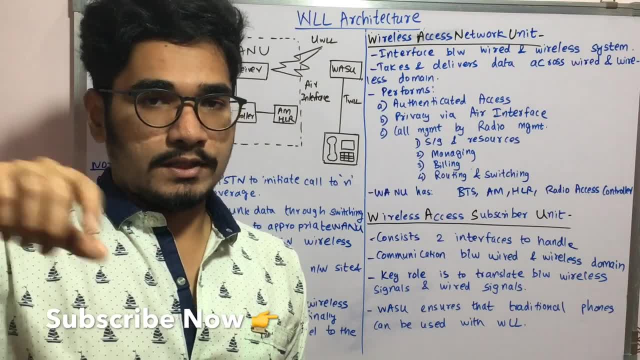 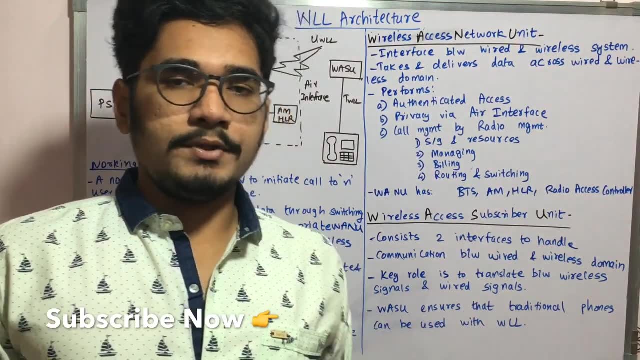 old phones where you had that ring kind of setup where you used to dial a number with that ring. So all those devices or all those units can be used with this. So well, that was all regarding the WLL architecture in wireless technology. So hope you guys enjoyed. 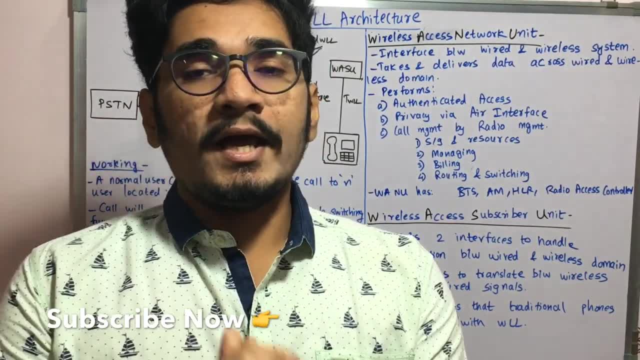 This will be fun. Thank you, guys, for watching this video. Please do like, share, comment and if you are new to this channel, please consider subscribing. Thank you very much for watching this video.